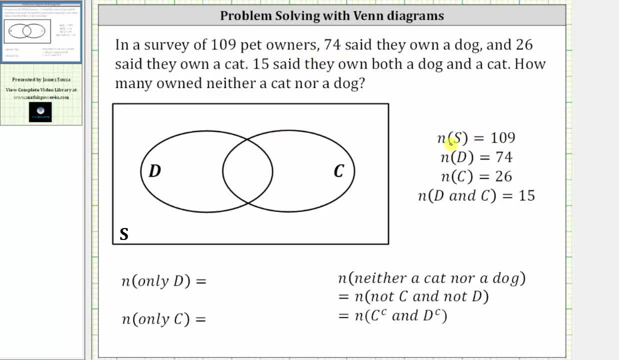 or the cardinality of set S is equal to 109, indicated using this notation. here, N of S equals 109.. And now, looking at the Venn diagram, we will let D equal the set of dog owners and C equal the set of cat owners. 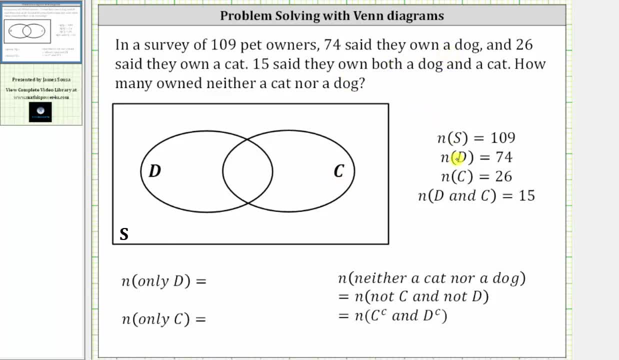 Because 74 said they own a dog, we know the number of elements in set D or the cardinality of set D is equal to 74.. 26 said they own a cat and therefore the number of elements in set Z is equal to 74.. 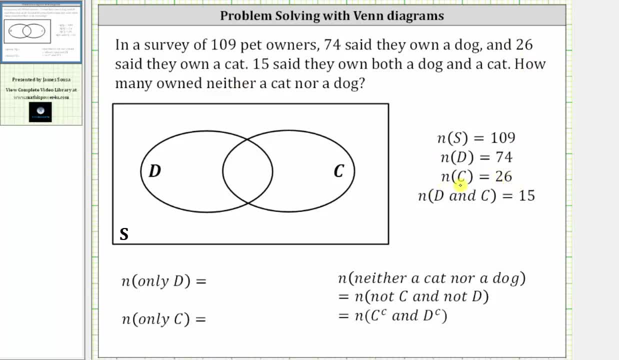 Set C is equal to 26,. or the cardinality of set C is equal to 26.. And finally, 15 said they own both a dog and a cat, which means the number of elements in set D and set C is equal to 15.. 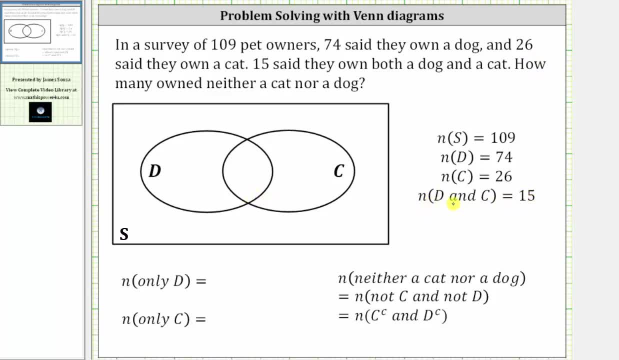 And now let's begin to label the Venn diagram. Because we know the number of elements in set D and set C is equal to 15, the intersection of set C and D must contain 15 elements. Let's go ahead and label this. 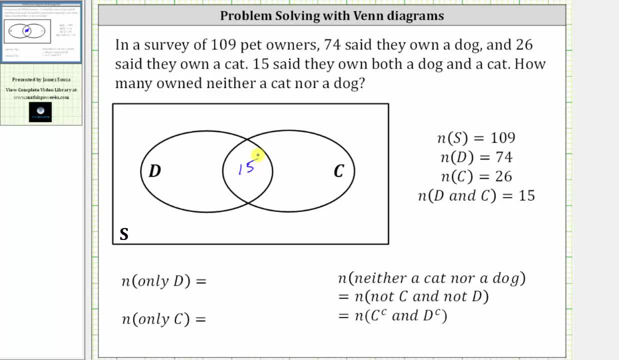 which would be the set here And now. before we can answer the question, we need to determine the number of elements that are only in set D, as well as the number of elements only in set C, Beginning with the number of elements only in set D. 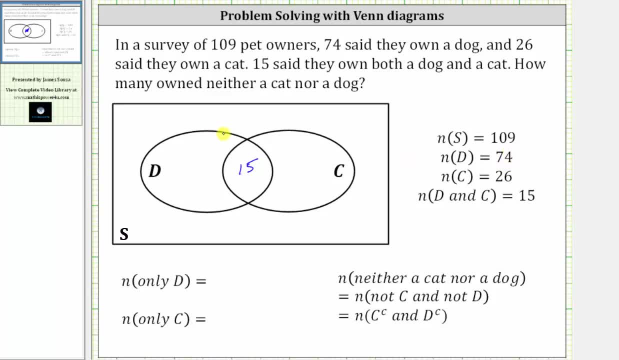 we know the number of elements in set D is equal to 74, but this is the set D And the set only D would be this set here. So, because we know there are 74 elements in set D, 15 of which are also in C. 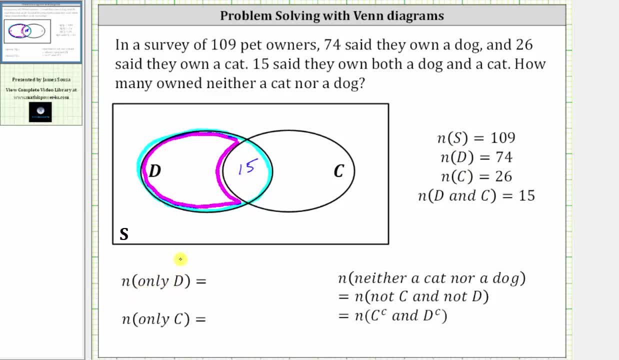 the number of elements only in set D is equal to 74,. the number of elements in set D minus the number of elements in set D and set C, which is 15.. 74 minus 15, is equal to 59. So there are 59 elements. 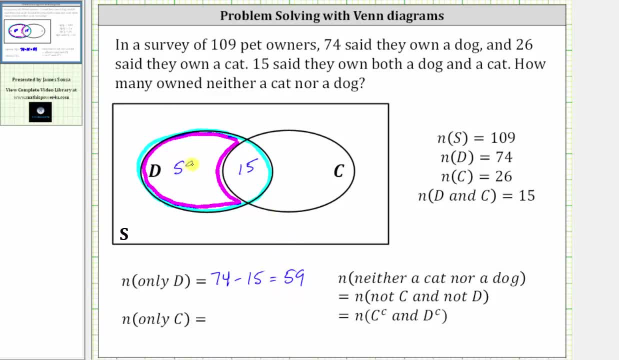 elements only in set D, which again is this set here in purple. And now to determine the number of elements that are only in set C, We are given there are 26 elements in set C. So here's set C. There are 26 elements in this set, The.